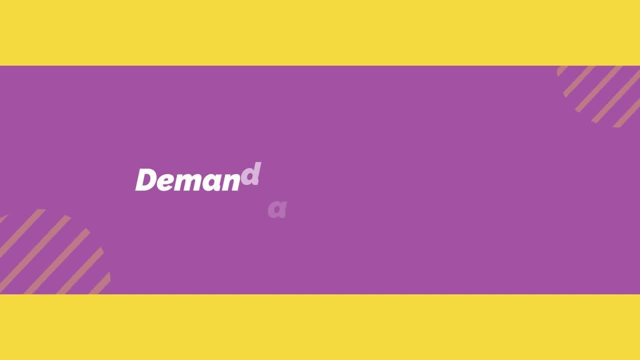 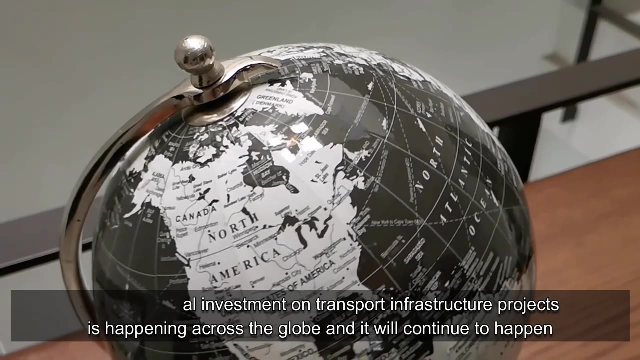 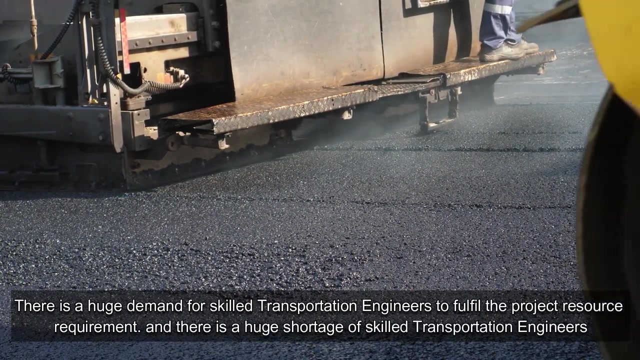 why transportation engineering a good career option? Demand and supply gap. Massive capital investment on transport infrastructure projects is happening across the globe and it will continue to happen. There is a huge demand for skilled transportation engineers to fulfill the project resource requirement And there is a huge shortage of skilled transportation engineers. 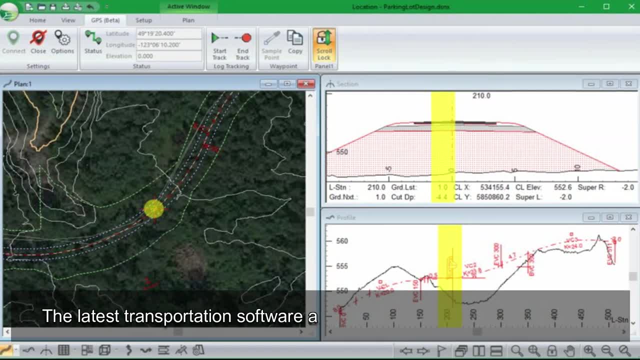 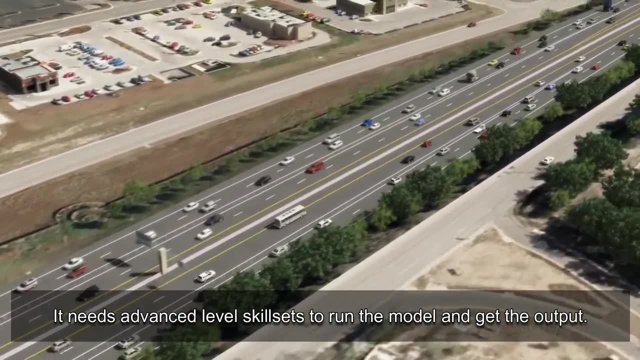 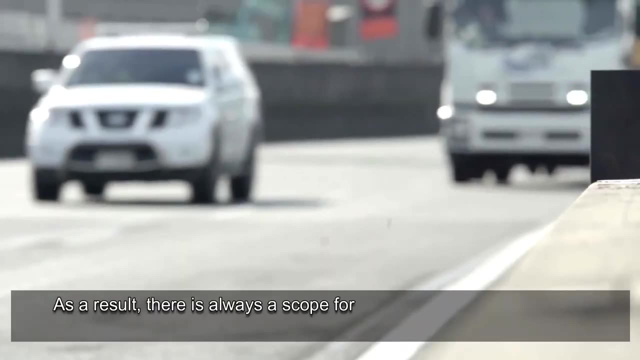 Complex tasks, complex technical skills. The latest transportation software and modeling tools are very complex. It needs advanced level skillsets to run the model and get the output Rapidly. changing technology Technology means you need to update yourself all the time. As a result, there is always a scope for 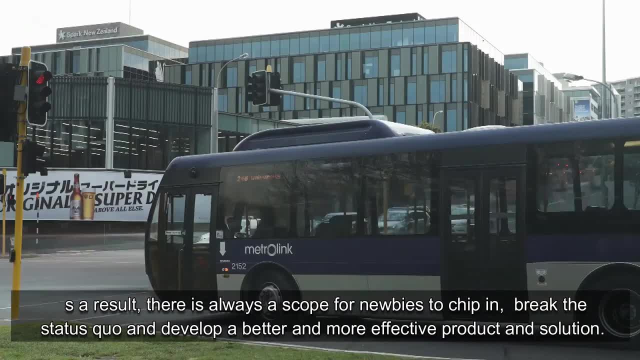 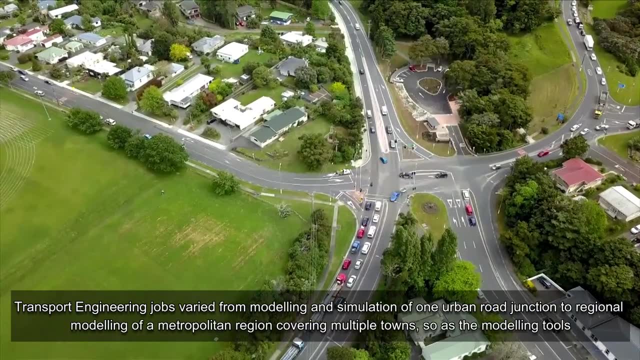 newbies to chip in, break the status quo and develop a better and more effective product and solution. Variation: Transport engineering jobs varied from modeling and simulation of one urban road junction to regional modeling of a metropolitan region covering multiple towns, so as the modeling 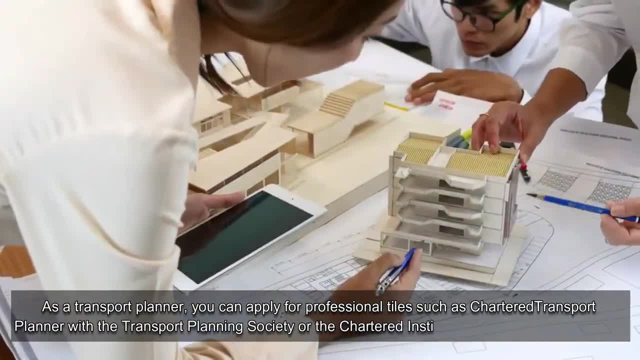 tools. As a transport planner, you can apply for professional tiles such as chartered transport planner. with the transport planner. You can apply for professional tiles such as chartered transport planner. with the transport planner. You can apply for professional tiles such as chartered transport. 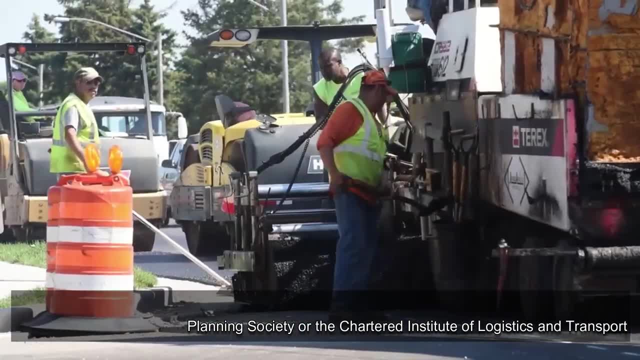 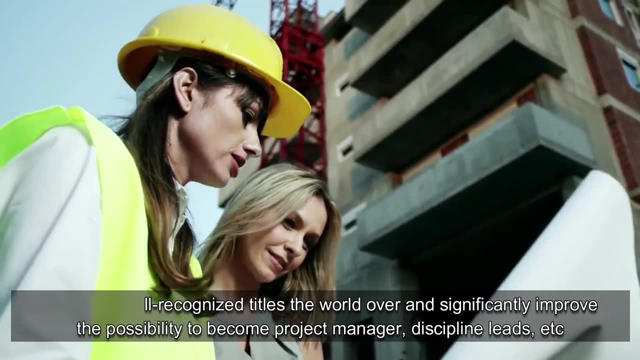 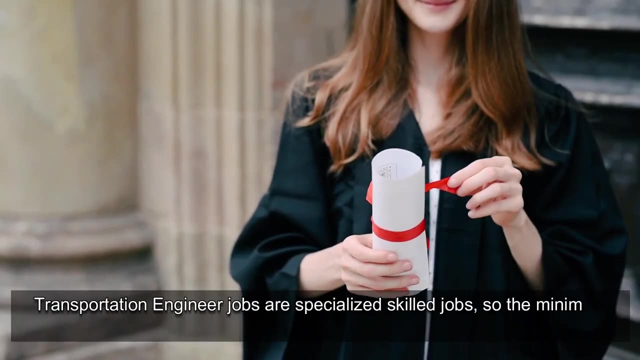 planning society or the chartered institute of logistics and transport. These are well-recognized titles the world over and significantly improve the possibility to become project manager, discipline leads, etc. Transportation engineer educational requirements. Transportation engineer jobs are specialized, skilled jobs, so the minimum requirement is a master's degree in transportation. 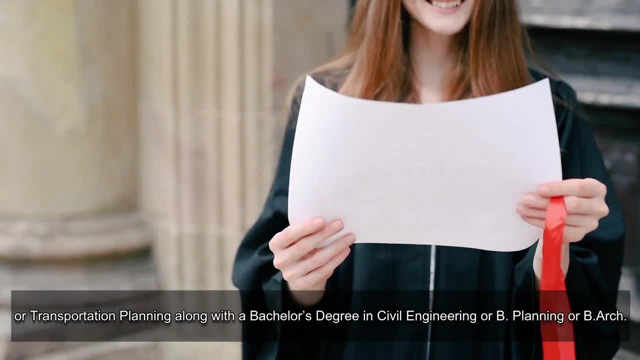 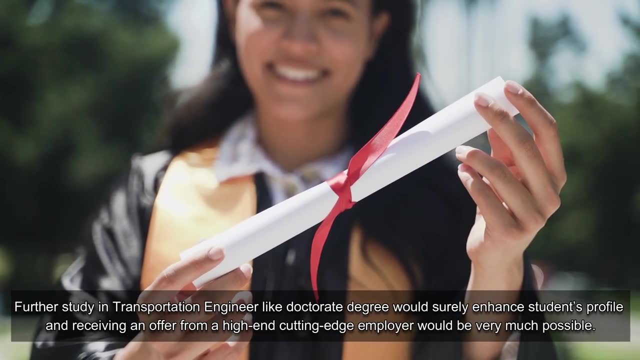 engineering or transportation planning, along with a bachelor's degree in civil engineering or be planning or be arch. Further study in transportation engineer-like doctorate degree would surely enhance student's profile and receiving an offer from a high-end, cutting-edge employer would be very much possible. 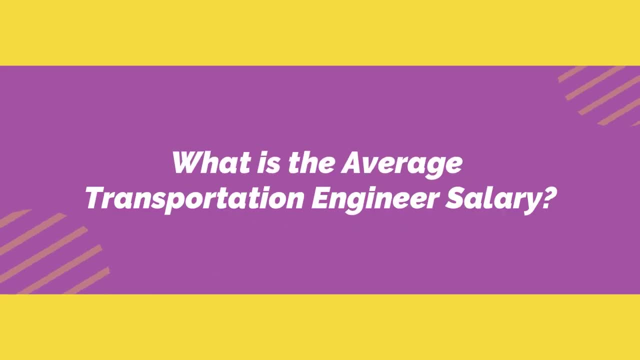 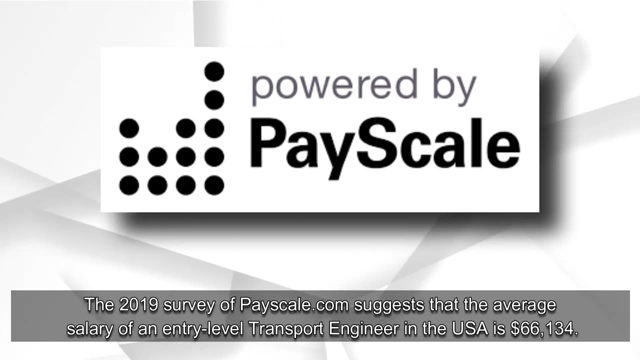 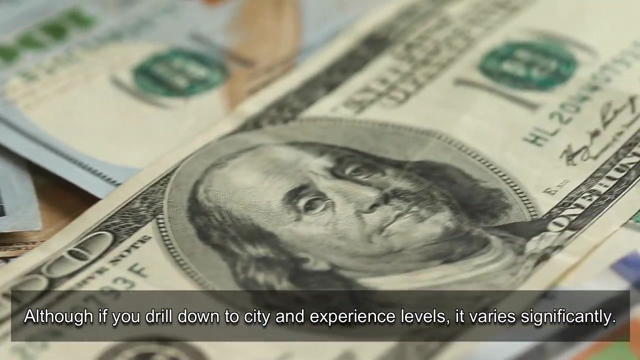 What is the average transportation engineer salary? The 2019 survey of payscalecom suggests that the average salary of an entry-level transport engineer in the USA is $66,134.. Although, if you drill down to city and experience levels, it varies significantly. 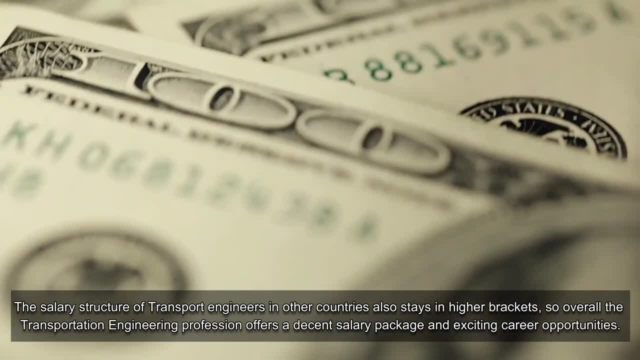 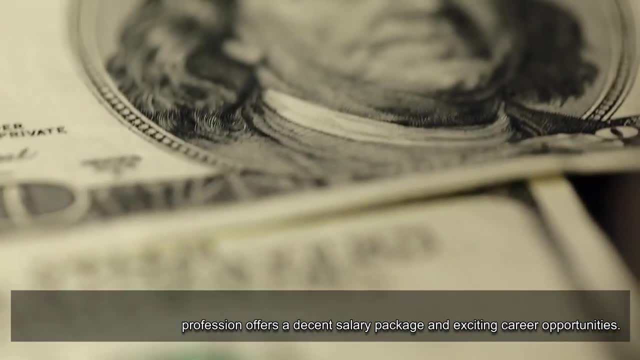 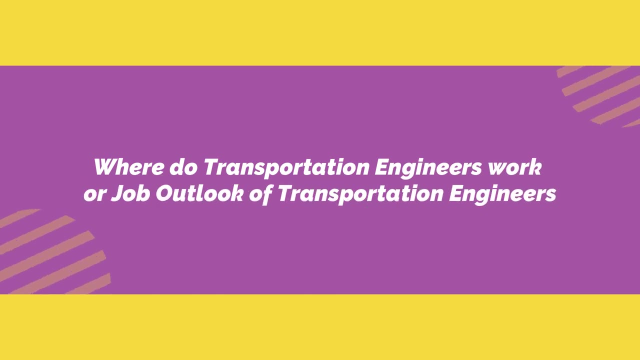 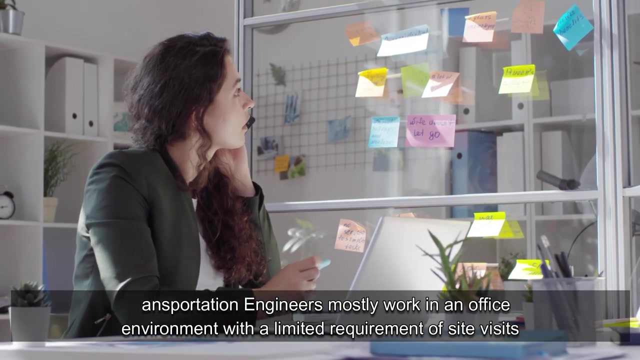 The salary structure of transport engineers in other countries also stays in higher brackets. so overall, the transportation engineering profession offers a decent salary package and exciting career opportunities. Where do transportation engineers work or job outlook of transportation engineers. Transportation engineers mostly work in an office environment with a limited requirement. 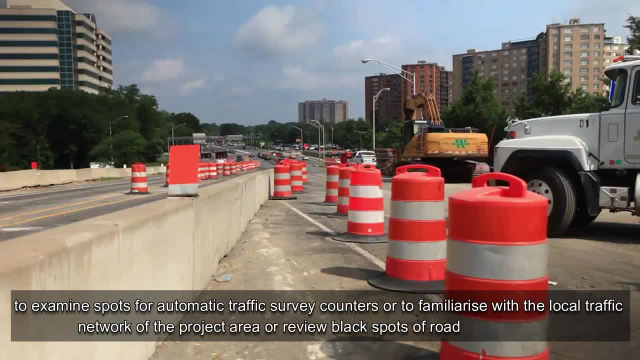 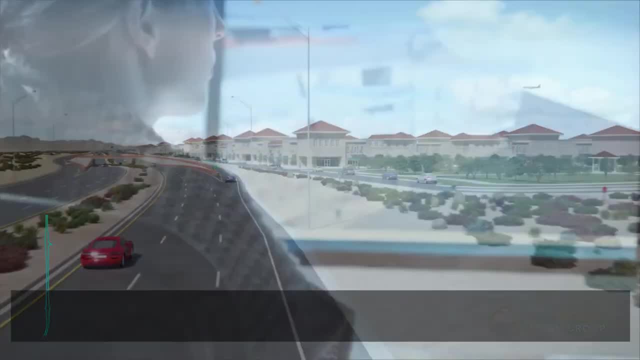 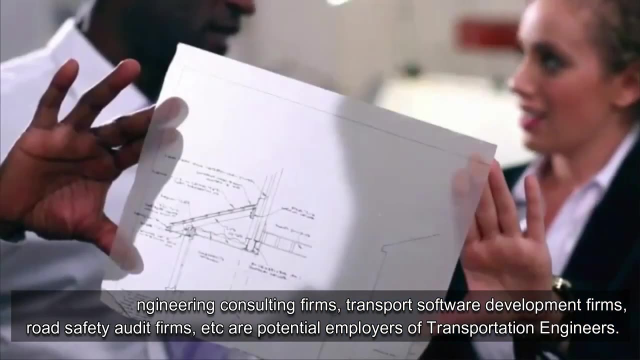 of site visits to examine spots for automatic traffic survey counters or to familiarize with the local traffic network of the project area or review black spots of road accidents, etc. Transportation engineering consulting firms, transport software development firms, road safety audit firms, etc. are potential employers of transportation engineers. 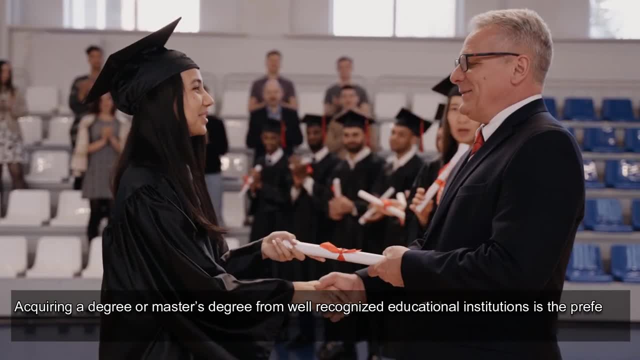 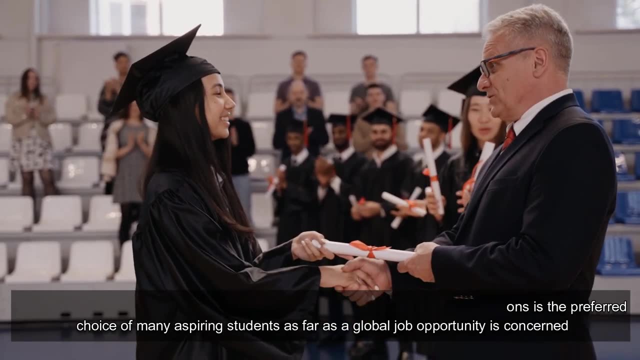 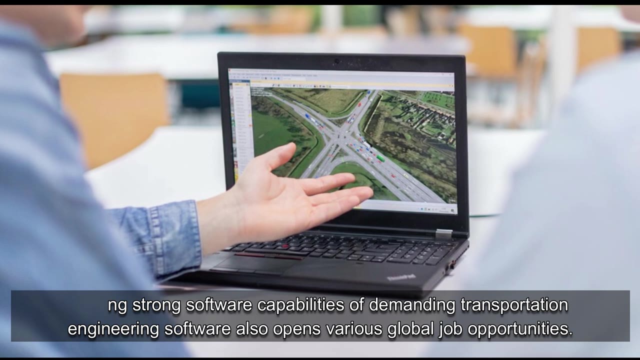 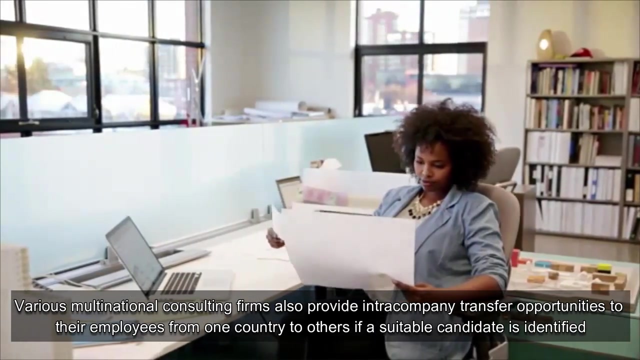 Global job opportunities. Acquiring a degree or master's degree from well-recognized educational institutions is the preferred choice of many aspiring students as far as the job opportunities are concerned. Having strong software capabilities of demanding transportation engineering software also opens various global job opportunities. Various multinational consulting firms also provide intra-company transfer opportunities. 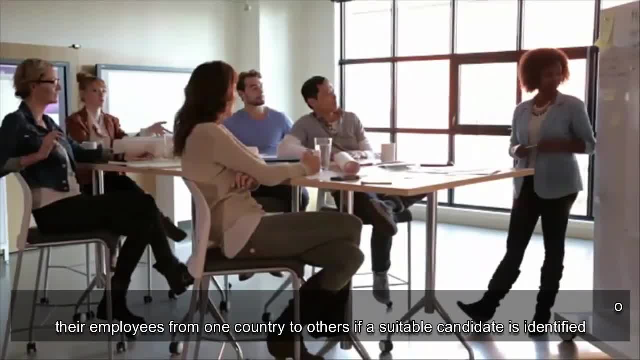 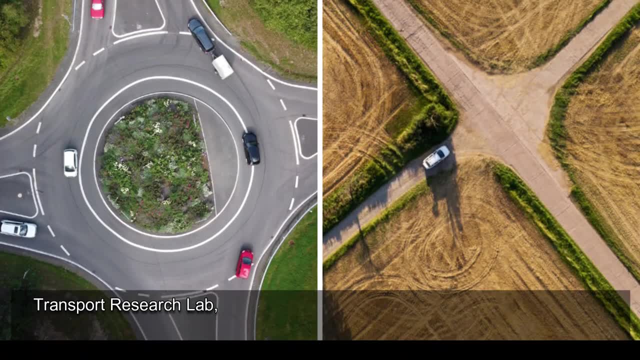 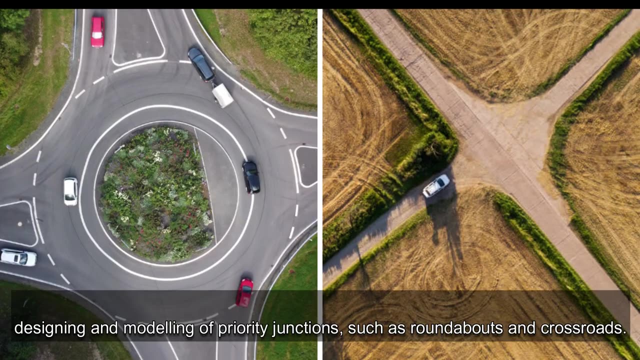 to their employees from one country to others if a suitable candidate is identified. Key transportation engineering softwares, Junction and signal design. Transport Research Lab UK provides Arcady, Picardy and Oscardy for the designing and modeling of priority junctions such as roundabouts and crossroads. 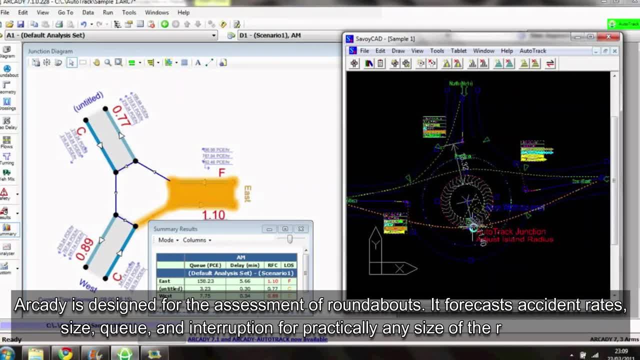 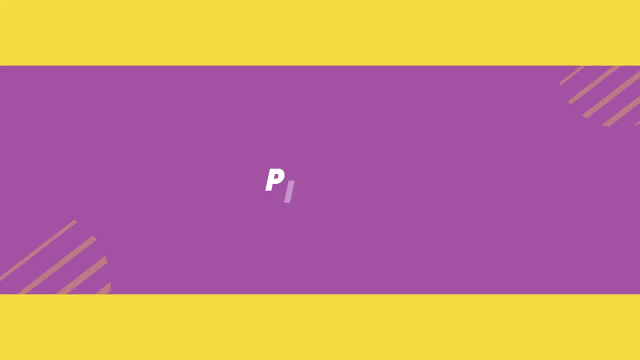 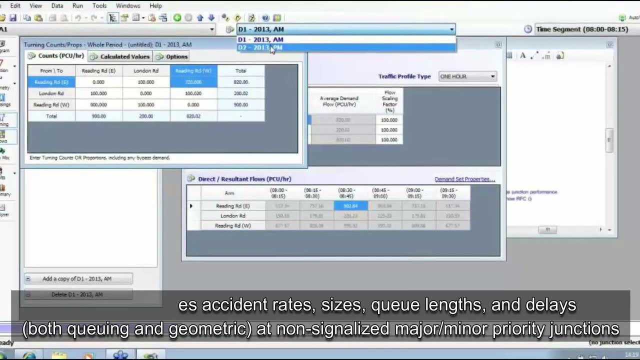 Arcady. Arcady is designed for the assessment of roundabouts. It forecasts accident rates, size, queue and interruption for practically any size of the roundabout Picardy. Picardy envisages accident rates, sizes, queue lengths and delays, both queuing and geometric, at non-signalized major-minor priority junctions. 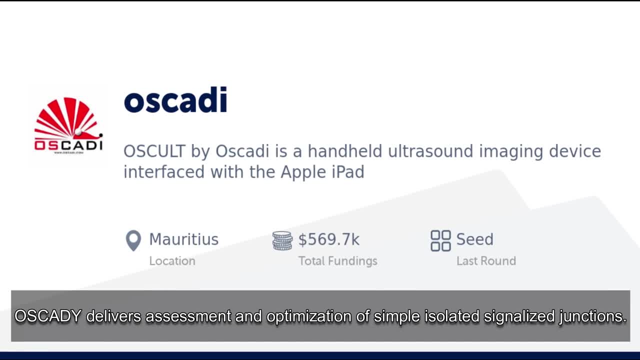 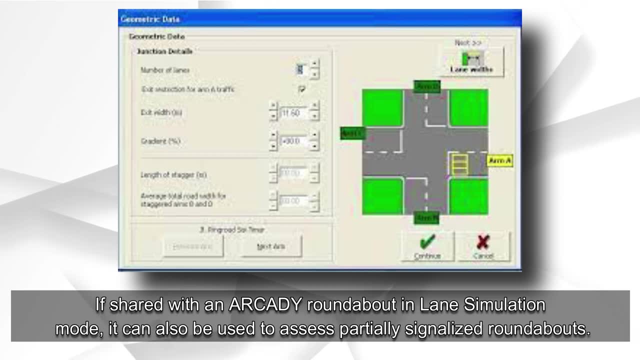 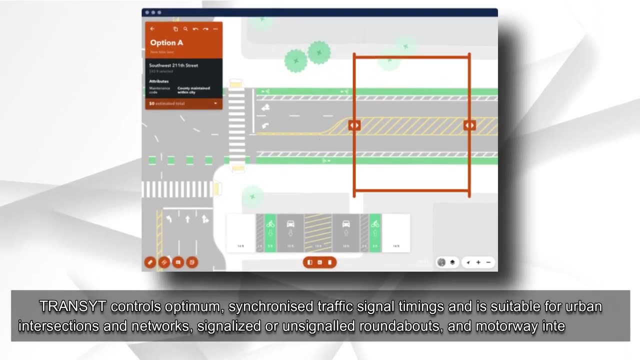 Oscardy. Oscardy delivers assessment and optimization of simple ISOs isolated signalized junctions. If shared with an Arcady roundabout, in lane simulation mode, it can also be used to assess partially signalized roundabouts. Transit Transit controls. optimum synchronized traffic signal timings. 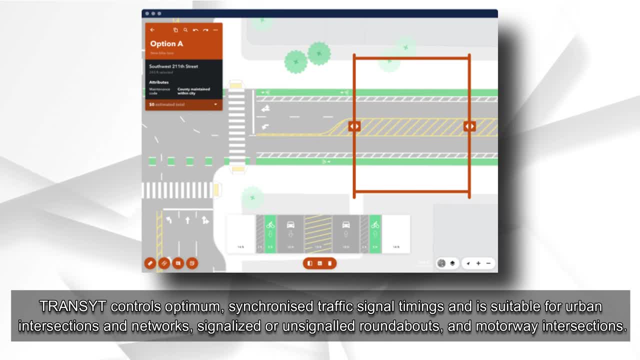 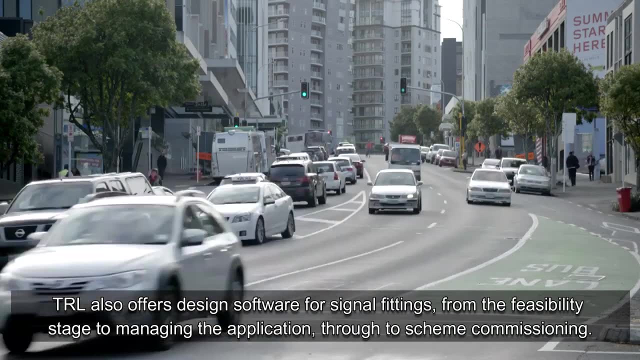 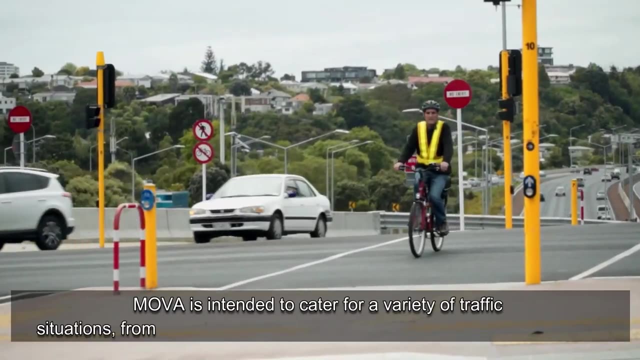 and is suitable for urban intersections and networks, signalized or unsignaled roundabouts and motorway intersections. Traffic Control TRL also offers design software for signal fittings, from the feasibility stage to managing the application through to scheme commissioning. Mova is intended to cater for a variety of traffic situations. 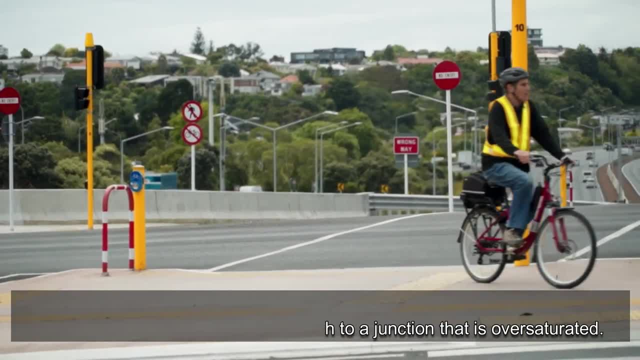 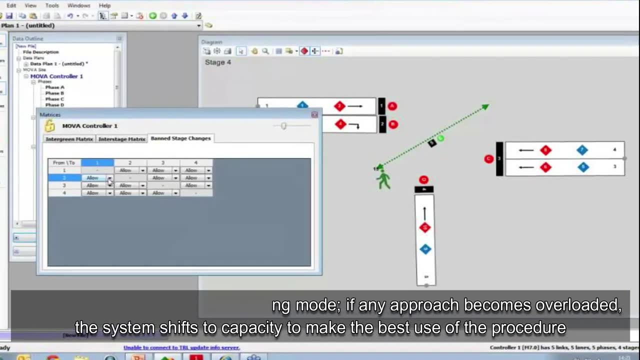 from very low flows through to a junction that is oversaturated. Mova operates in a delay-minimizing mode. If any approach becomes overloaded, the system shifts to capacity to make the best use of the procedure. Scoot is an actual and competent solution. 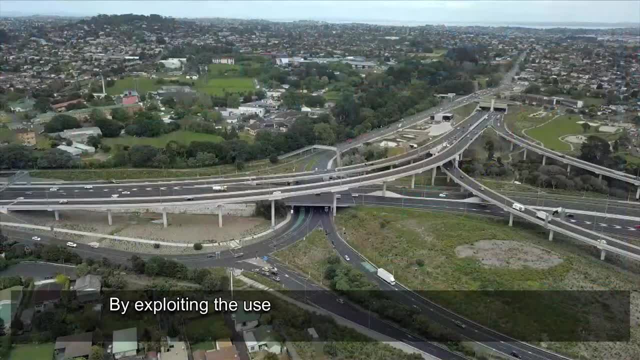 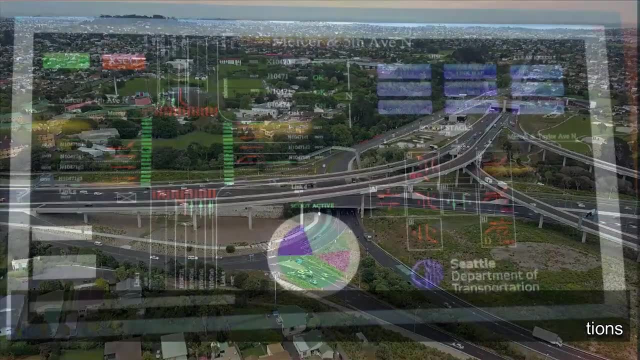 for controlling traffic on signalized road networks. By exploiting the use of live data from vehicle sensors, Scoot rapidly regulates traffic signal settings to reduce vehicle interruption. Scoot replies rapidly to changes in traffic, but not so fast that it is wobbly. 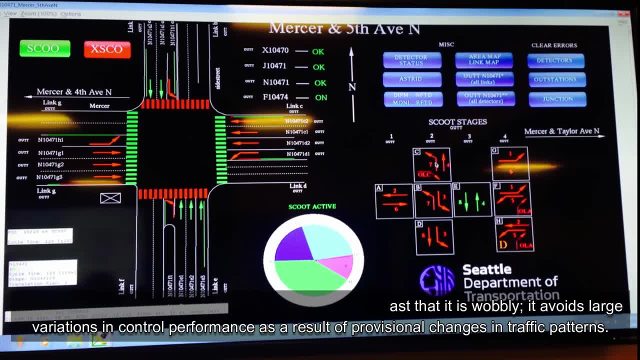 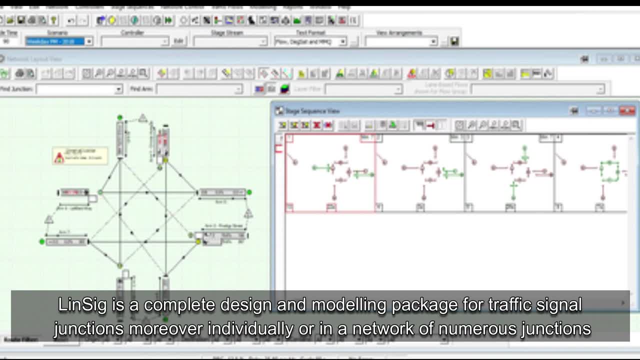 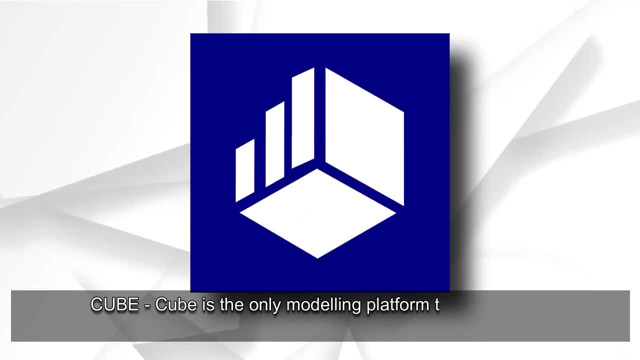 it avoids large variations in control performance as a result of provisional changes in traffic patterns. Linsave is a complete design and modeling package for traffic signal junctions, moreover, individually or in a network of numerous junctions, Transport Planning and Land Use. CubeCube is the only modeling platform. 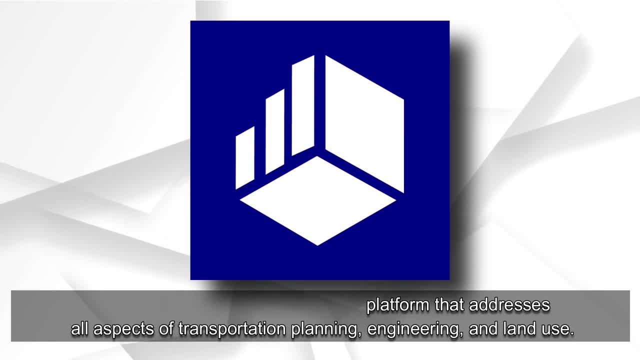 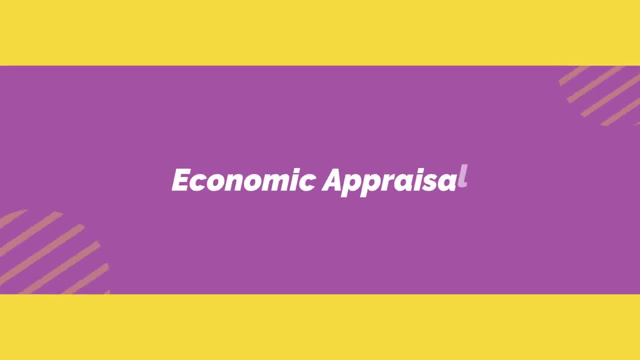 that addresses all aspects of transportation, planning, engineering and land use. With an up-to-date system, with an open platform, Cube allows to size and regulate models of any type. Economic Appraisal, HDM-4- The Highway Design and Maintenance Standards Model. 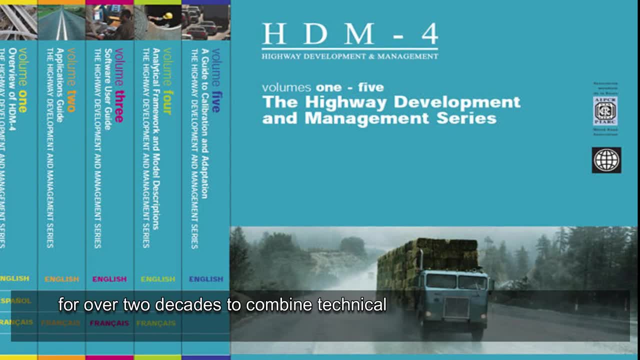 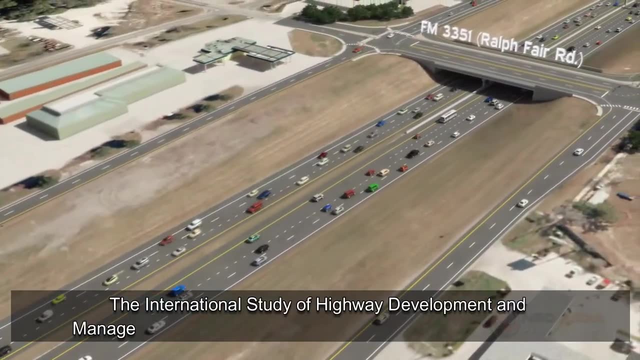 HDM-IRI, developed by the World Bank, has been used for over two decades to combine technical and economic appraisal of road investment projects, standards and strategies. The International Study of Highway Development and Management, ISINGDEM, has extended the scope of the HDM-IRI model. 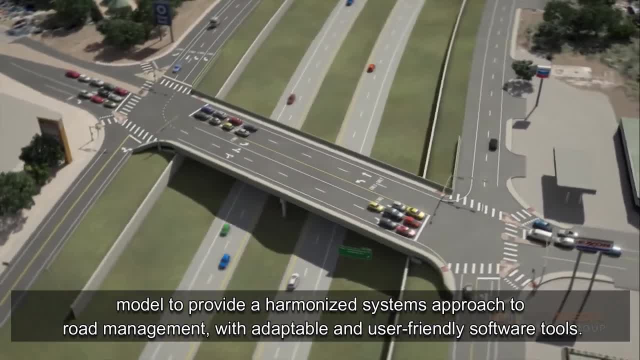 to provide a harmonized systems approach to road management with adaptive and efficient road management. The HDM-IRI model is a well-designed model for road management and is a well-designed model for road management. The HDM-IRI model is a well-designed model for road management. 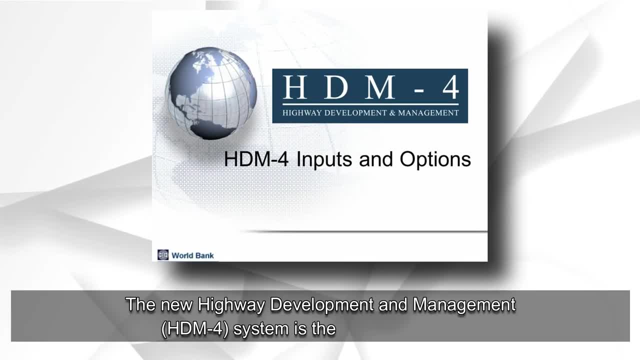 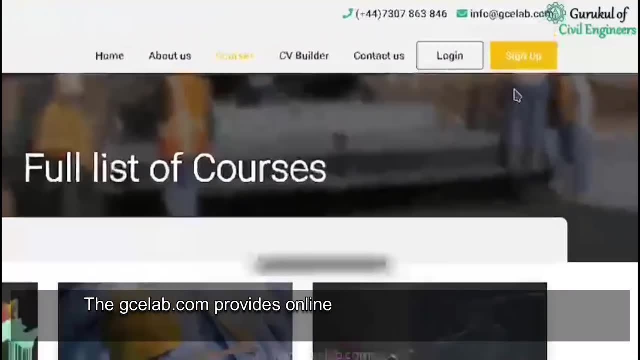 and is a well-designed model for road management, and is a well-designed model for road management and user-friendly software tools. The new Highway Development and Management HDM-IV system is the result of the study Online Courses. The gclubcom provides online courses. 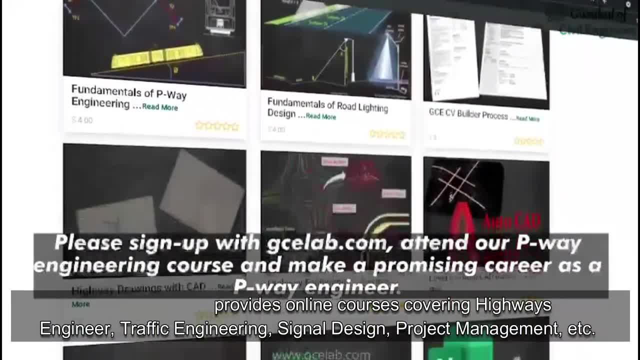 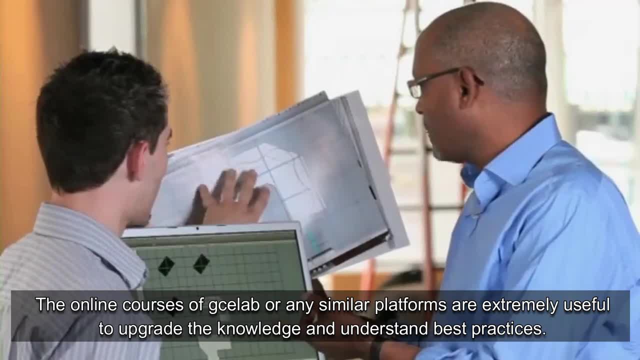 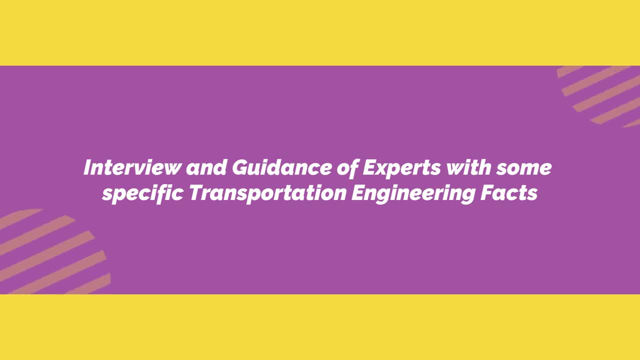 covering highways engineer, traffic engineering, signal design, project management, etc. The online courses of gclub or any similar platforms are extremely useful to upgrade the knowledge and understand best practices, Interview and guidance of experts with some specific transportation engineering engineering facts. 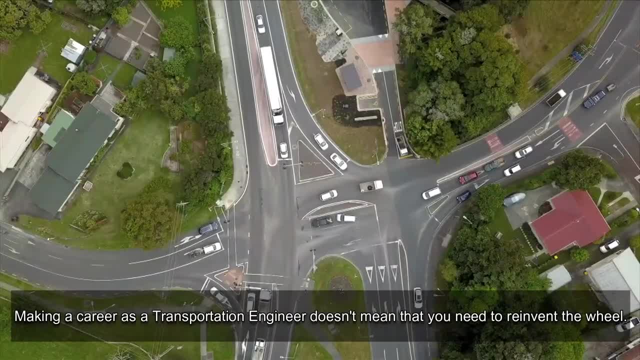 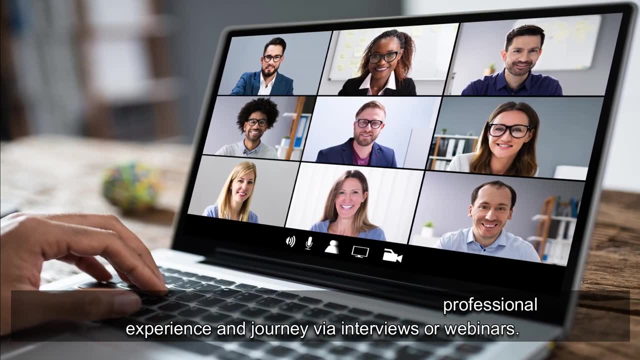 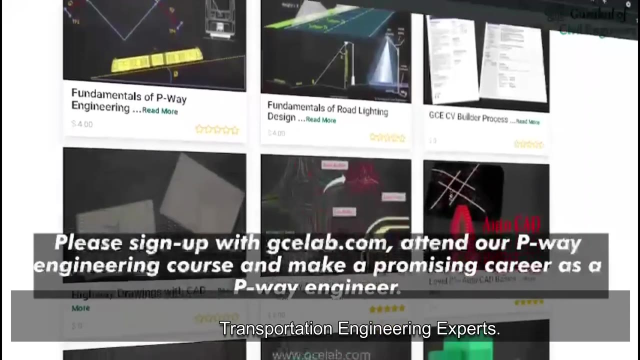 Making a career as a transportation engineer doesn't mean that you need to reinvent the wheel. Various experts across the globe share their professional experience and journey via interviews or webinars. The gclubcom also talks to various industry experts, including transportation engineering experts. 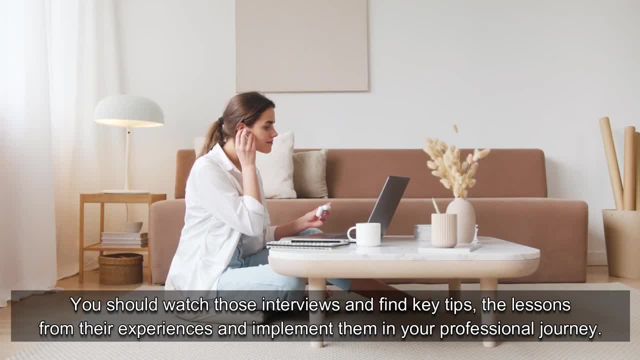 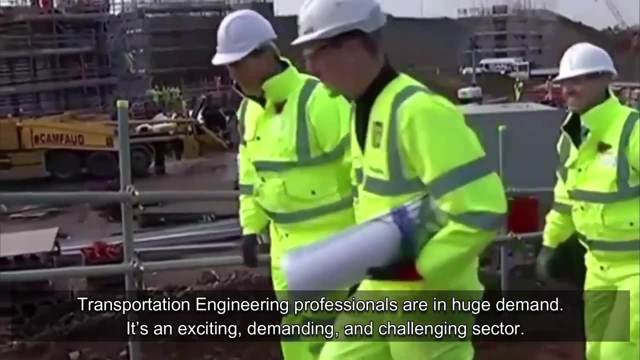 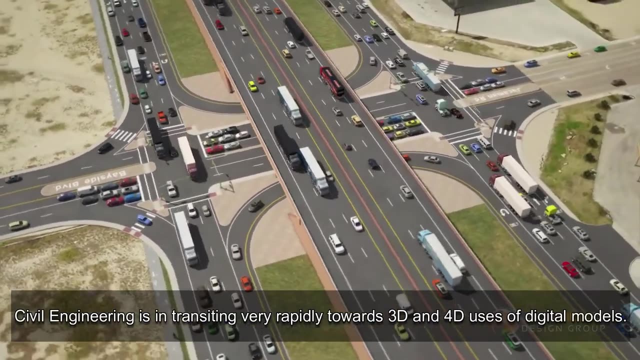 You should watch those interviews and find key tips, the lessons from their experiences and implement them in your professional journey. Key takeaways: Transportation engineering professionals are in huge demand. It's an exciting, demanding and challenging sector. Civil engineering is in transiting very rapidly. 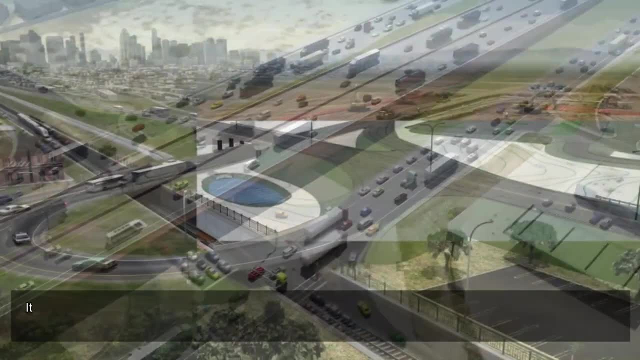 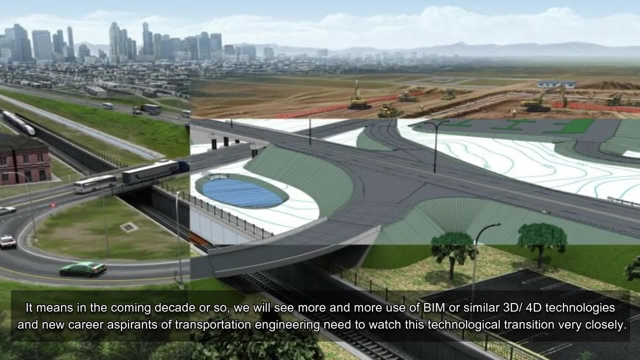 towards 3D and 4D uses of digital models. It means in the coming decade or so we will see more and more use of BIM or similar 3D, slash, 4D technologies, and new career aspirants of transportation engineering need to watch this technological transition very closely. 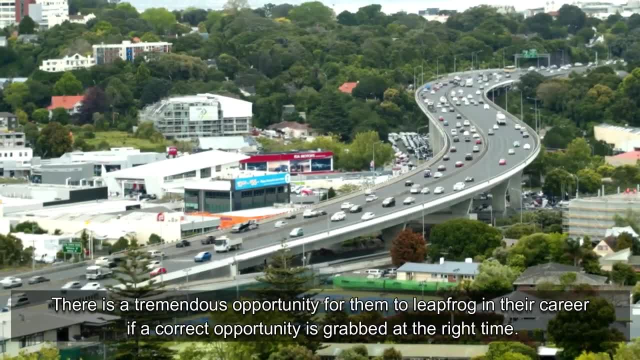 There is a tremendous opportunity for them to leapfrog in their career If a correct opportunity is grabbed at the right time. Feel free to like, share and comment. 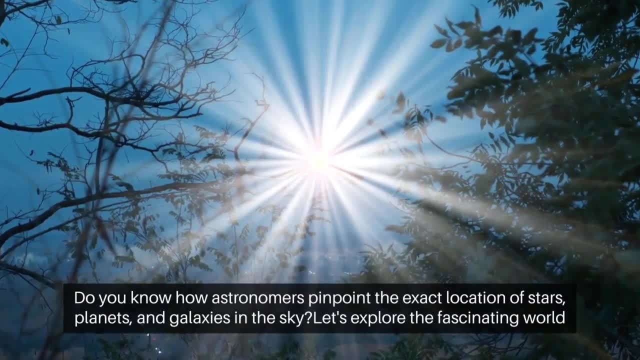 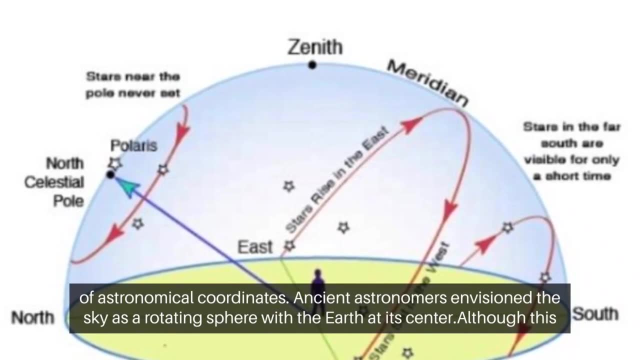 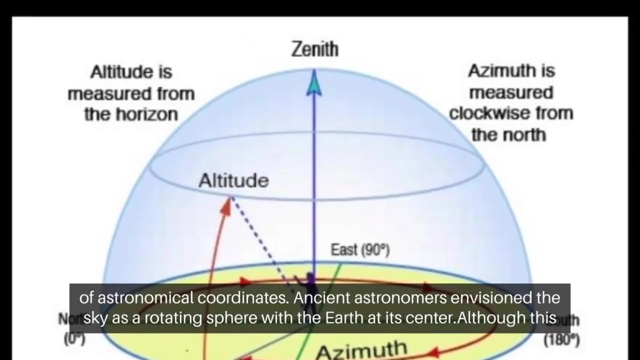 Do you know how astronomers pinpoint the exact location of stars, planets and galaxies in the sky? Let's explore the fascinating world of astronomical coordinates. Ancient astronomers envisioned the sky as a rotating sphere with the Earth at its center. Although this concept isn't real, it remains a useful tool for astronomers. 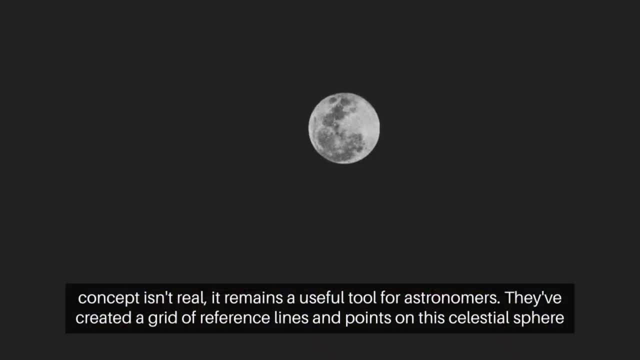 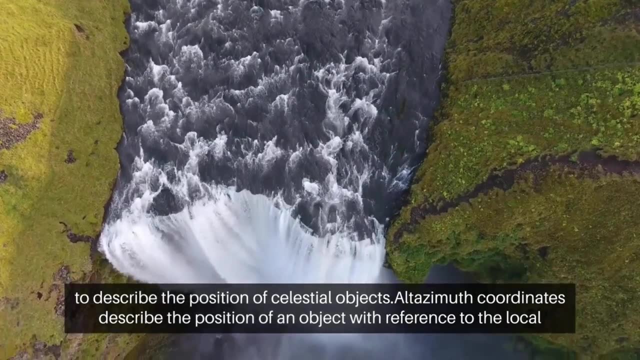 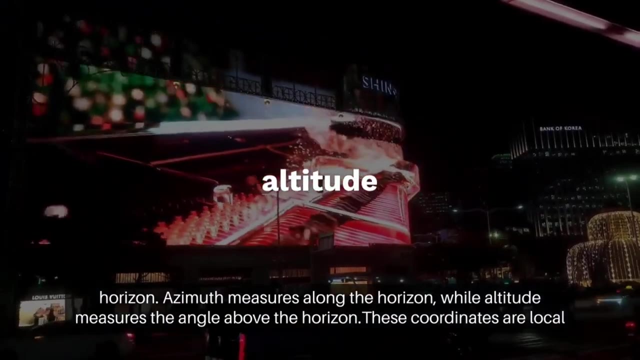 They've created a grid of reference lines and points on this celestial sphere to describe the position of celestial objects. Alt-azimuth coordinates describe the position of an object with reference to the local horizon. Azimuth measures along the horizon, while altitude measures the angle above the horizon. 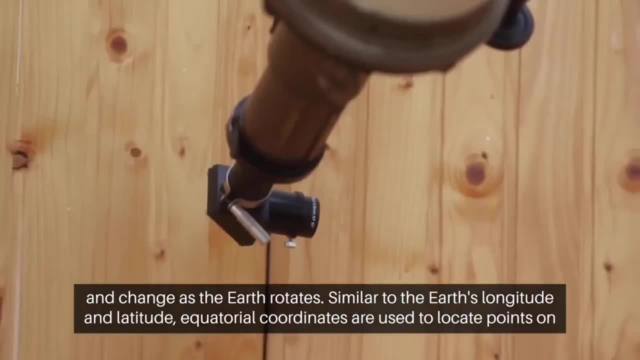 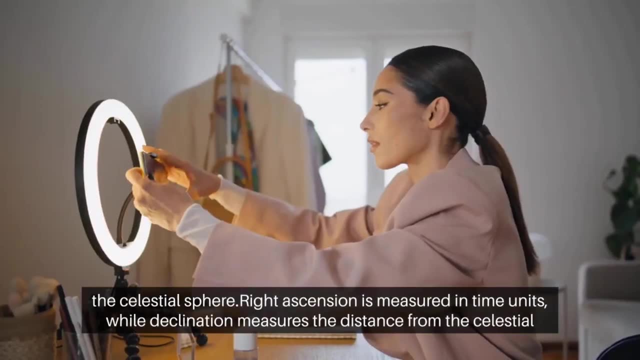 These coordinates are local and change as the Earth rotates, Similar to the Earth's longitude and latitude. equatorial coordinates are used to locate points on the celestial sphere. Right ascension is measured in time units, while declination measures the distance from the celestial equator. 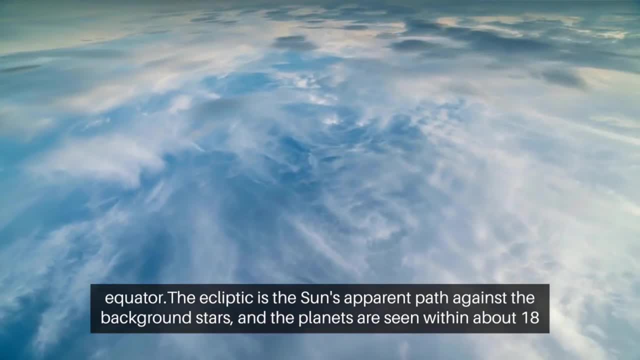 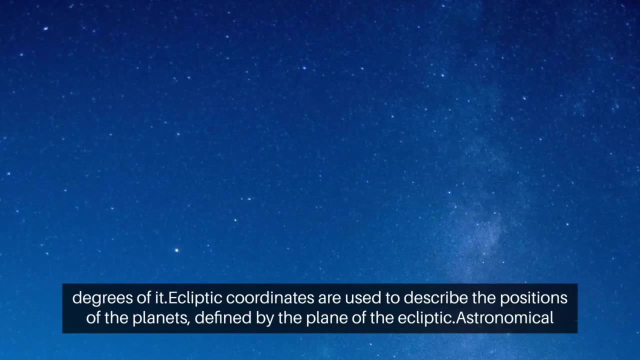 The ecliptic is the Sun's apparent path against the background. stars and the planets are seen within about 18 degrees of it. Ecliptic coordinates are used to describe the positions of the planets defined by the plane of the ecliptic. 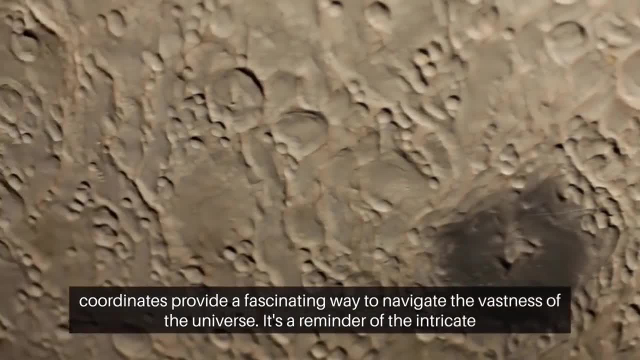 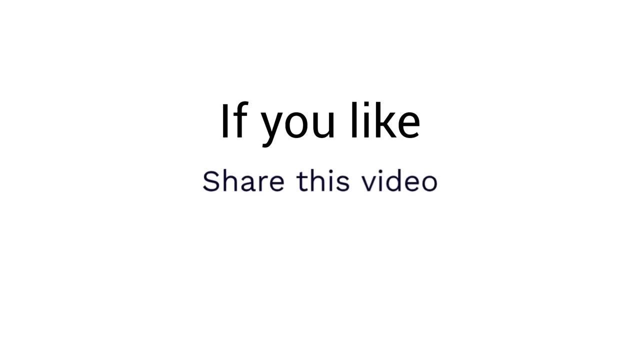